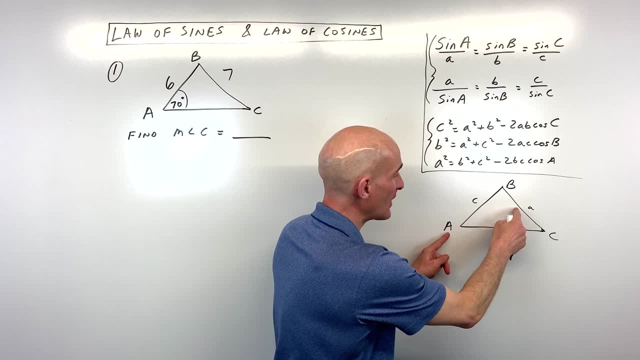 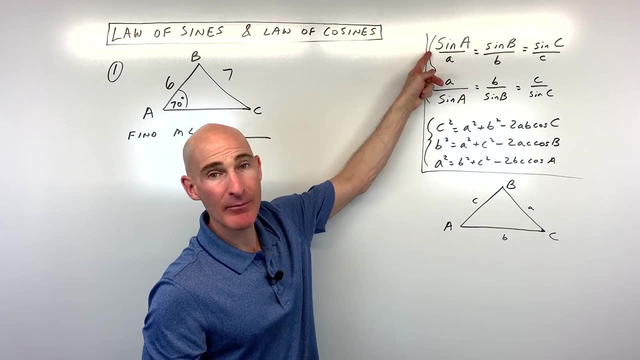 side lengths And notice that here's angle A across from angle a is side A, across from angle b is side b, across from angle c is side c. And when we do the law of sines, I like to use this top equation here You can think of this ratio: the sign of angle a over its side opposite That ratio. is equal to the sine of angle a, precious, and that ratio is equal to the sin of the angle a. or do I use theseaster, orX, xprs, the harmonica of angle a, bleaching over the Stevens and the lefthand? 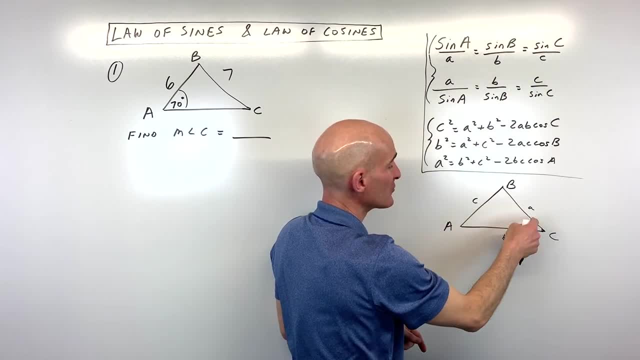 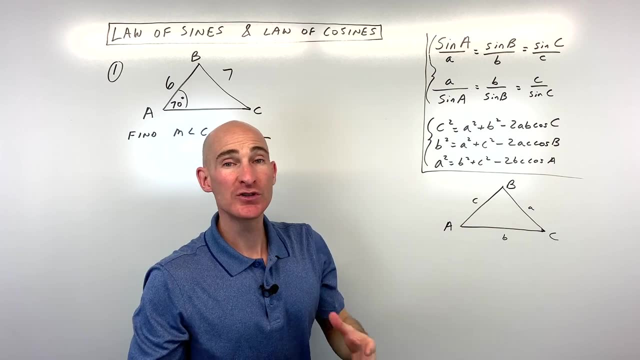 of angle B over its side opposite, and that's equal to the ratio of sine of angle C over its side opposite. So you only need to use two of these three ratios to form a proportion, and then you can solve for the missing quantity. What I like to think of is: I like to think: 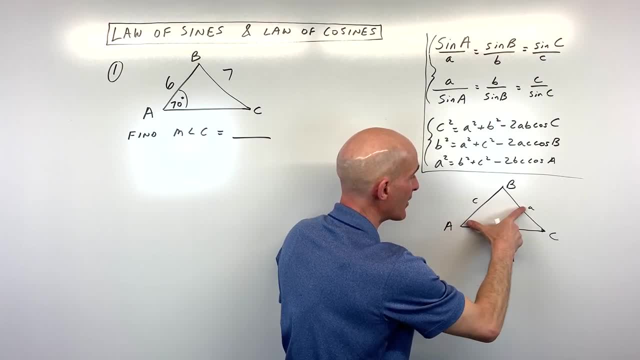 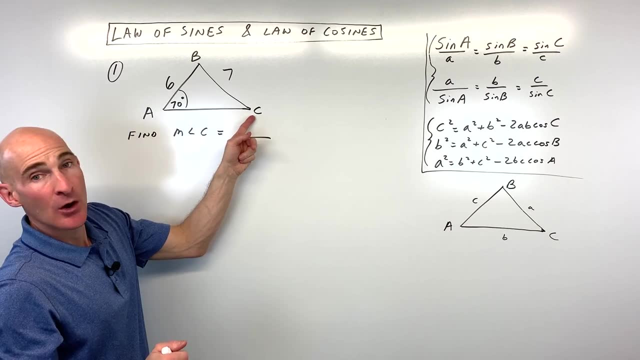 of the angle and the side across as like a pair. So you've got a pair, a pair and a pair like that. So let me show you the first example. Like say, here we want to find the measure of angle C. Well, what I notice first off is that I have 70 degrees and I have the 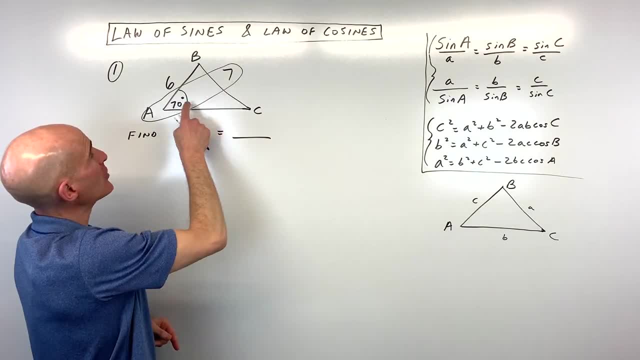 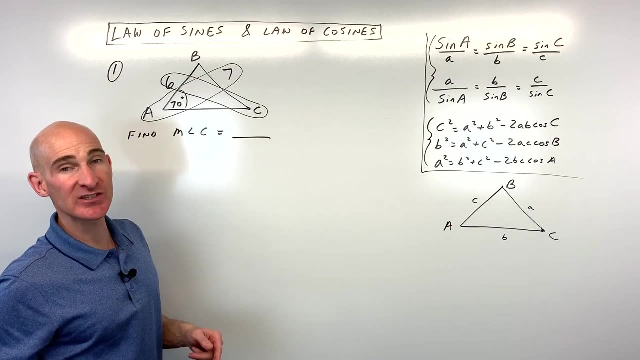 side, across from that 70 degree angle. I also have this side here, 6, and I'm looking for angle C, which is across from this side length of 6.. So basically, what we have is we have two pairs and so we only have one unknown quantity, angle C. So what I'm going to do? 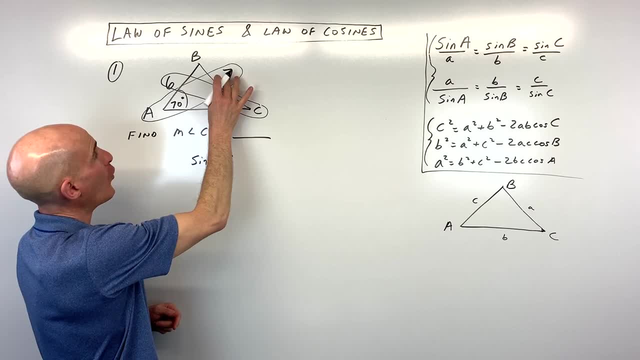 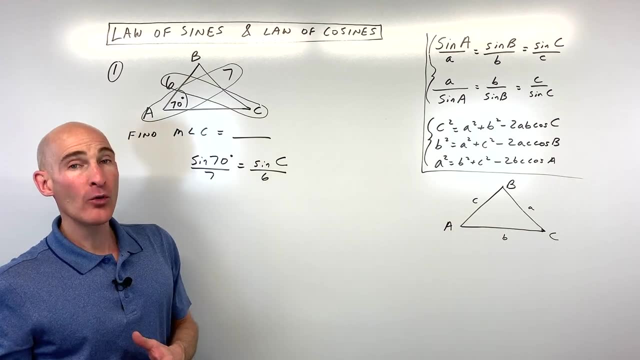 is. I'm going to say the sine of 70 degrees over its side opposite equals the sine of angle C Over its side opposite, which is 6.. Now, all we have to do now is we need to get sine of angle C by itself. So I'm going to multiply both sides by 6.. That way, the numerator and 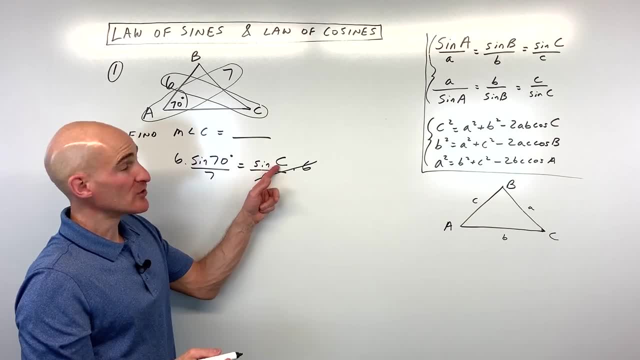 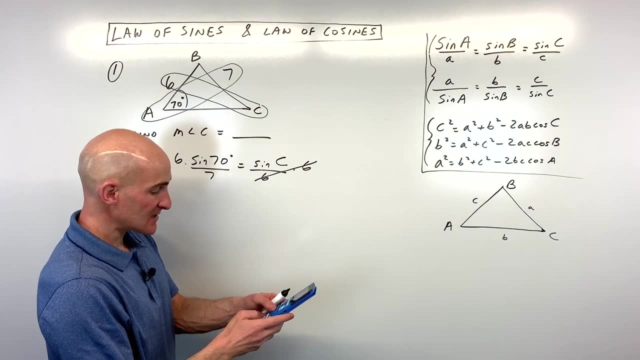 denominator cancel. And then what we're going to do to solve for angle C is we're going to have to take the sine inverse of this quantity. Let's do it one step at a time, though. So first things first. we've got 6 times the sine of 70 degrees all divided by 7, and that comes. 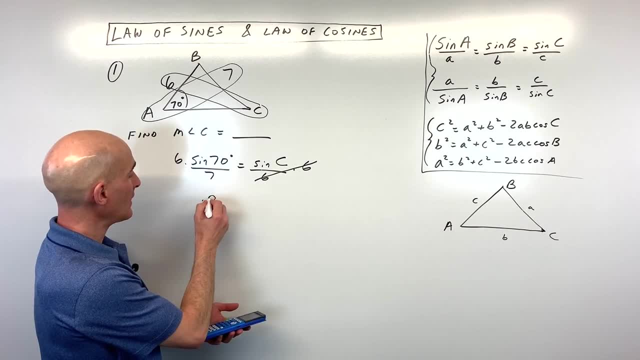 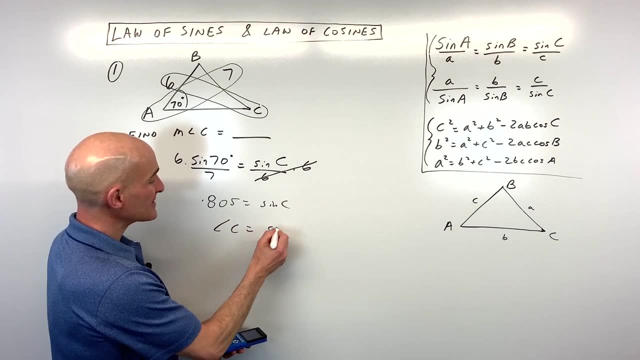 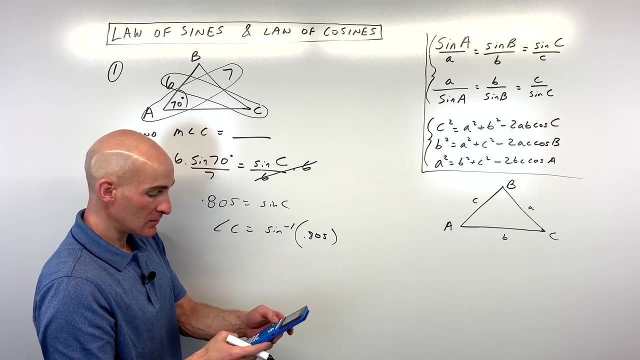 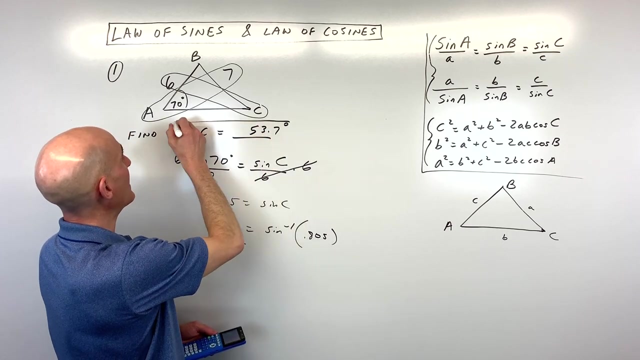 out to about .805.. So .805.. If we want to solve for angle C, we're going to do the sine inverse of .805, and let's see what that comes out to: 53.7 degrees. So let's write that here, 53.7 degrees, and you've got. 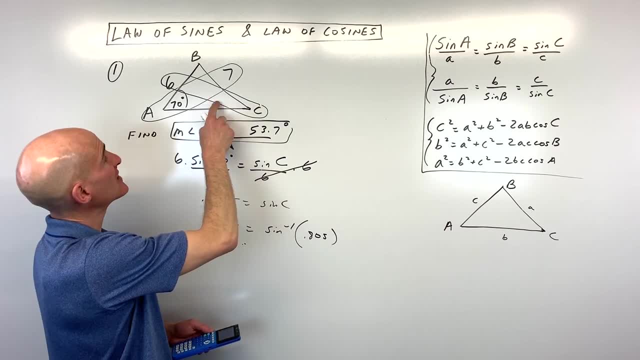 it. That's the measure of angle C. Now, if you want to proceed from there, then you can say: well, I know these two angles. I can subtract from 180 to find this angle. I could do law of sines again to find this missing side. 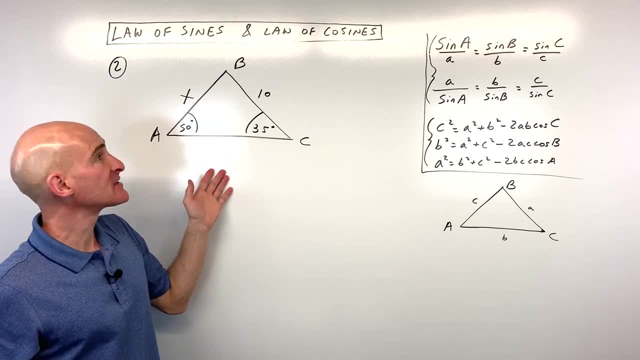 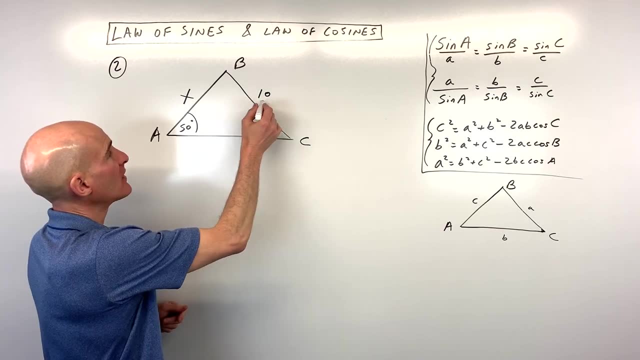 And then you've solved the triangle. Okay, our second example: using the law of sines, we're trying to find this missing side right here, X and again, what we want to do is we want to think about the angle and the side across from that angle as like a pair. So here we've. 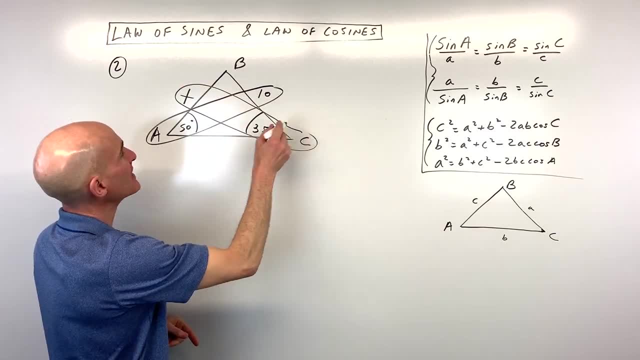 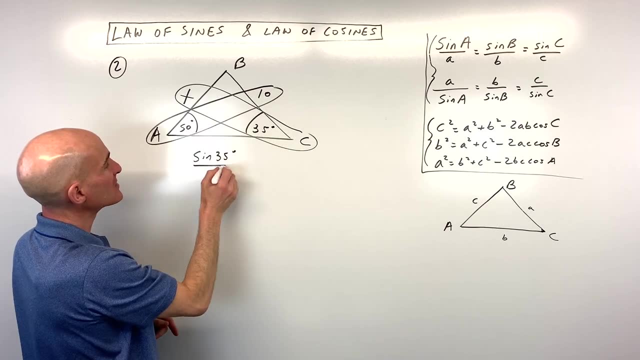 got 50 degrees and 10. here we have 35 degrees and x, So we can use our law of sines to solve for this missing a quantity. We've got: sine of 35 degrees over its side opposite equals sine of 50 degrees over its side opposite. 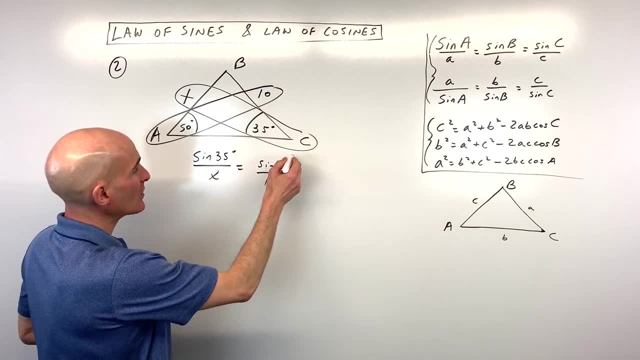 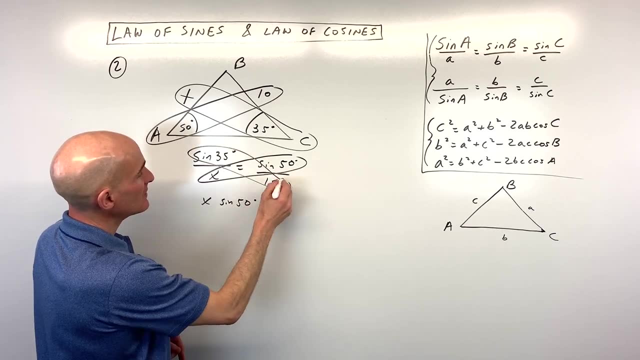 And now all we have to do is get this variable by itself. Now what we can do is we can cross, multiply x times. the sine of 50 degrees equals 10 times the sine of 35 degrees. Now all we have to do instead of multiplying by sine of 50. 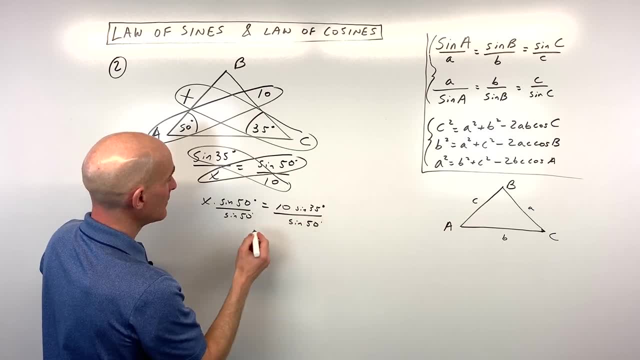 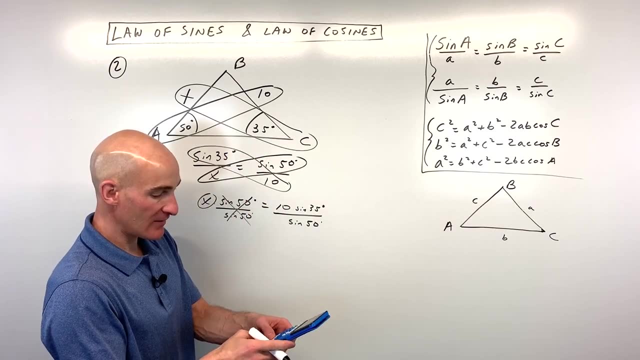 is: divide both sides by sine of 50 degrees. That gives us x by itself and we can calculate that length. So let's go ahead and do that. We've got 10 sine of 35 divided by sine of 50.. Make sure your calculator is in degree mode. 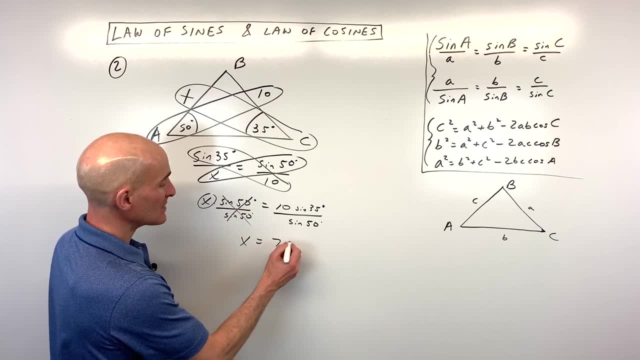 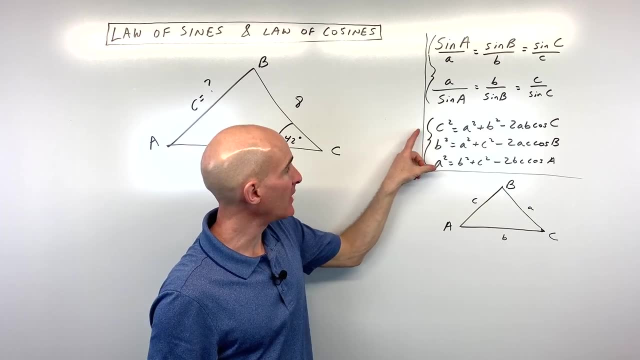 since we're working with degrees And it comes out to approximately 7.5.. And the next two examples: we're gonna talk about the law of cosines. We're gonna be working with these three formulas here at the bottom. Now, if you know one of these formulas, 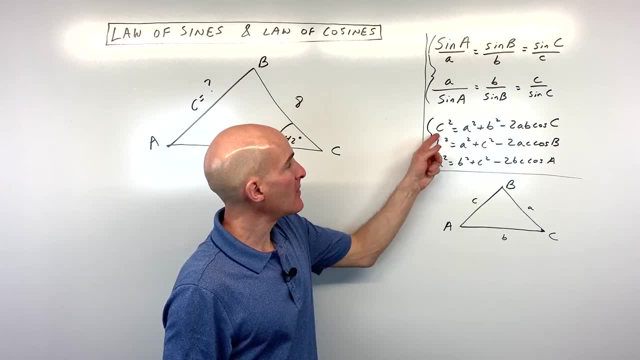 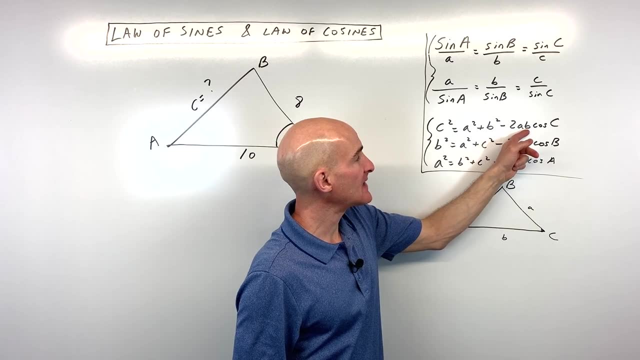 you'll automatically know the other two. So what I recommend is start off by memorizing this top one: c squared equals a squared plus b squared, just like Pythagorean theorem: minus two times a times b times the cosine of angle c. 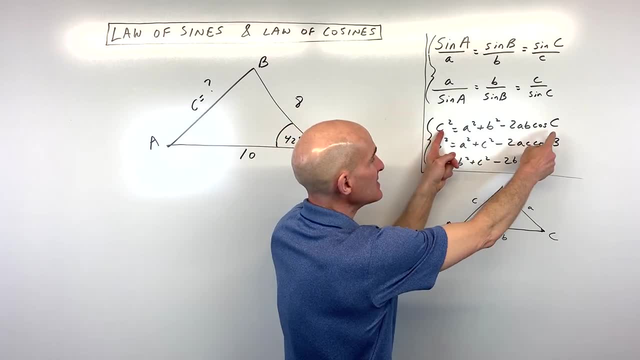 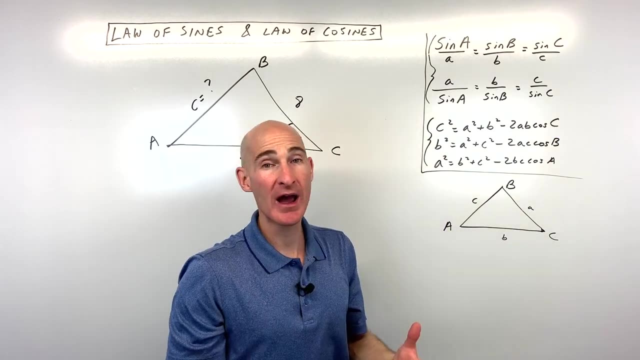 One thing you'll notice about these formulas is that see how this is side c and angle c. See how they're across from each other or at opposite ends in the formula, Just like they're across from each other in the triangle If we use this middle formula. see side b, angle b. 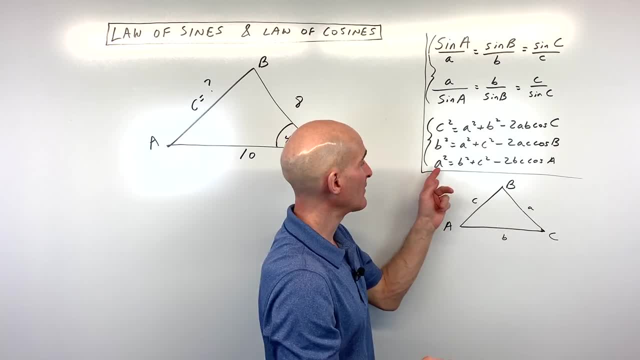 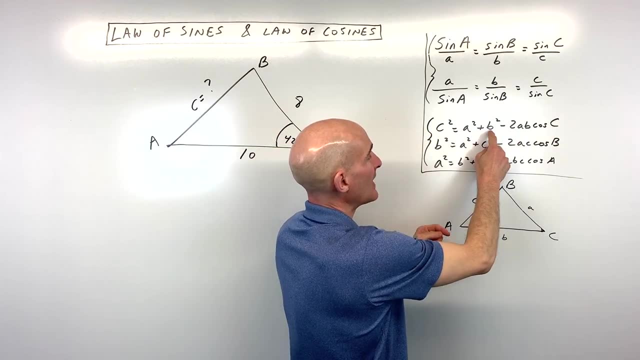 they're across from each other in the formula, they're across from each other in the triangle and we've got side a and angle a And notice, then if we're working with this top one, see c and c. then we've got a and b, a and b. 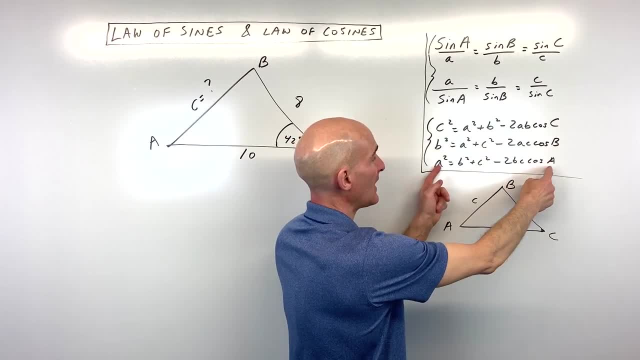 If we're working with b, we've got a and c, a and c. If we're working with a, we've got b and c, b and c- the other two that we're not using right. So when do we use law of cosines? 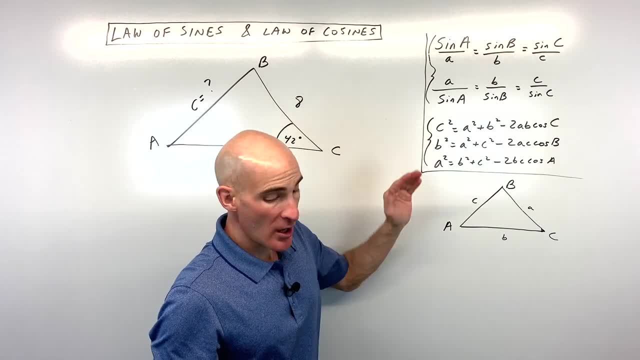 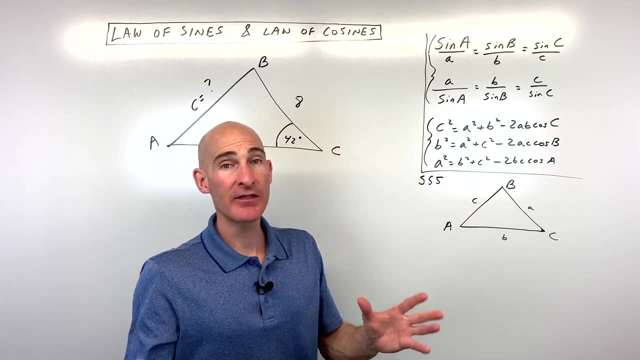 That's the question a lot of students ask. Well, you can use the law of cosines, okay, or you actually have to use the law of cosines when they only give you three sides, like side, side side, nothing else? 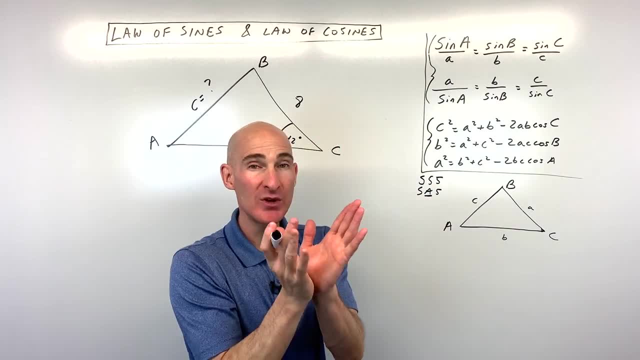 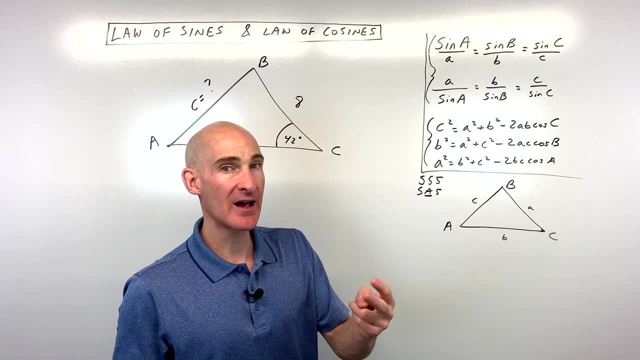 Or they give you side angle. side meaning the angles in between the two given sides. If you try to use law of sines, what'll happen is you have too many unknowns You won't be able to solve because you've got like two variables or more. 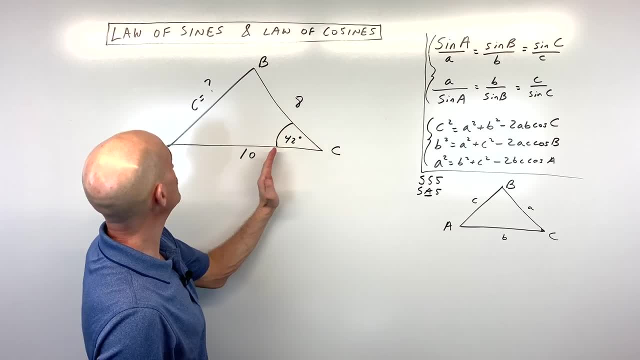 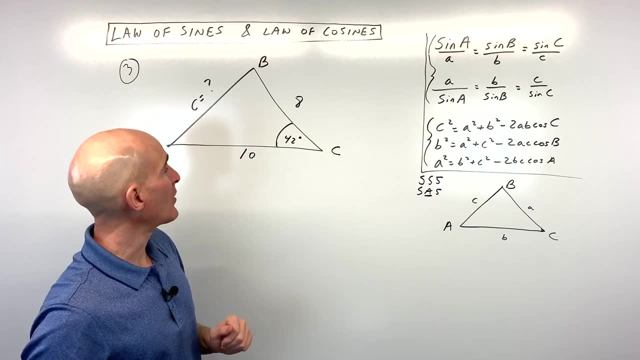 So that's when you use law of cosines Side side side or side angle side. Let me show you example number three here. Okay, notice what we have. We've got side angle side- That case I was talking about right here. 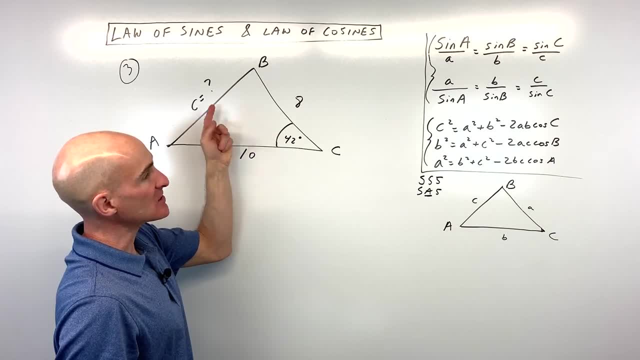 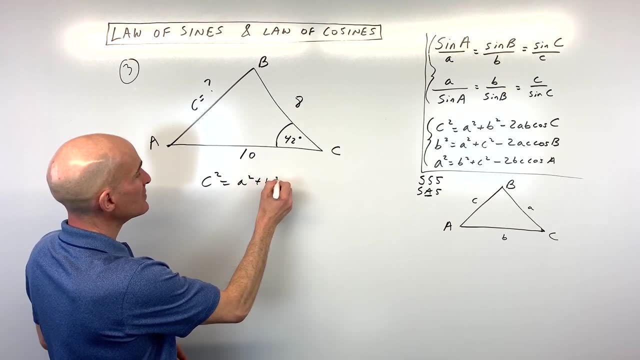 We wanna find the side across from angle c, side c. So we're gonna use this top formula here And let's go ahead and write it out. So we have c squared equals a squared plus b squared minus, two times a times b times the cosine of angle c. 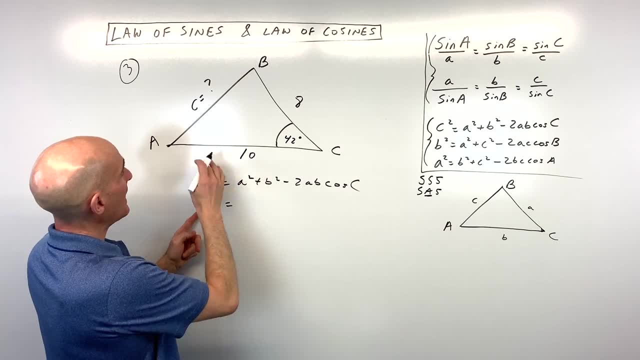 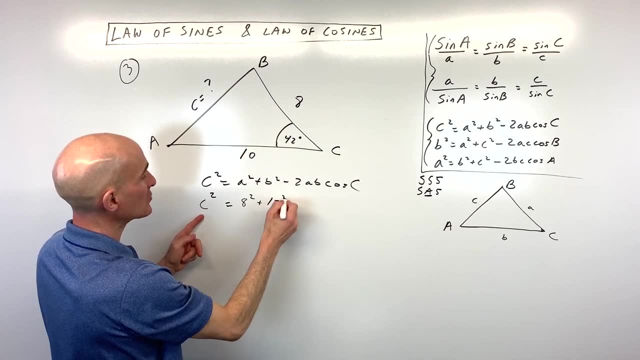 We don't know what c is, so let's just leave that as variable c. Okay, a is the side across from angle a. That's eight squared plus b. That's the side across from angle b. That's 10 squared minus two times eight times 10. 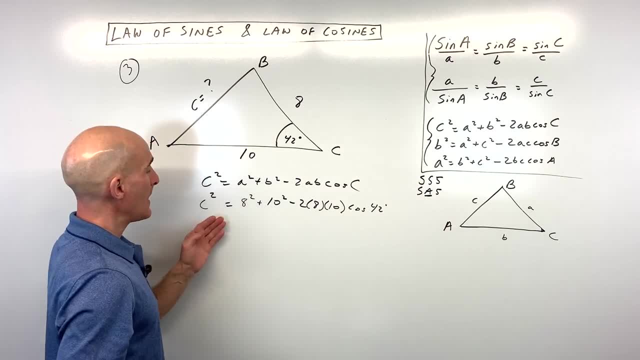 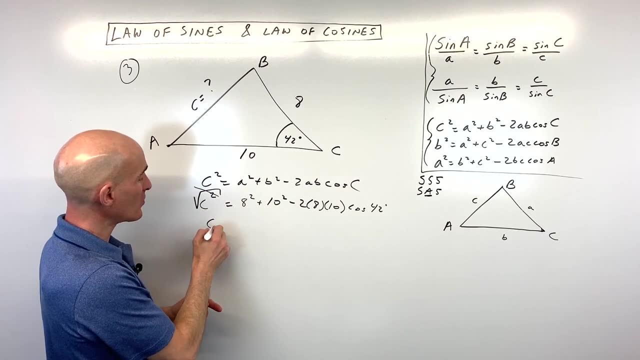 times the cosine of angle c, which is 42 degrees. Now notice how this is c squared here. We just wanna solve for side c, not c squared. So what I'm gonna do is I'm gonna take the square root, because the square and the square root. 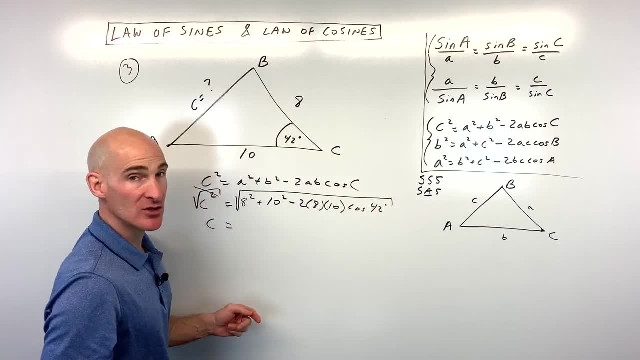 those are inverses. they cancel. If we do that to the left side, we also wanna do it to the right side. So let's go to our calculator, Let's put all that in and we're gonna take the square root. 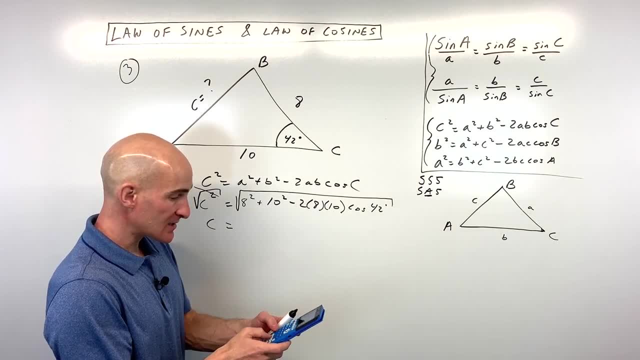 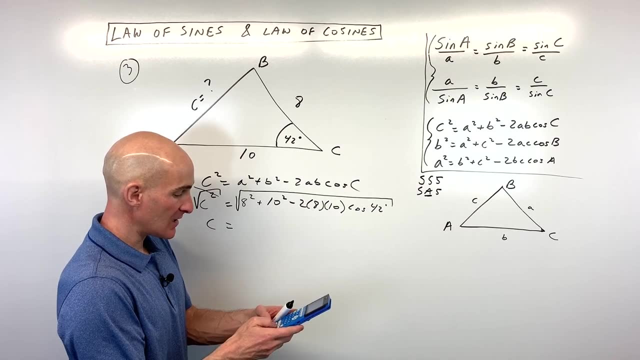 So if you use parentheses, you can take the square root. If you use parentheses, you can do all this in one step. Eight squared plus 10 squared: let's see minus two times, eight times, 10 times the cosine of 42.. 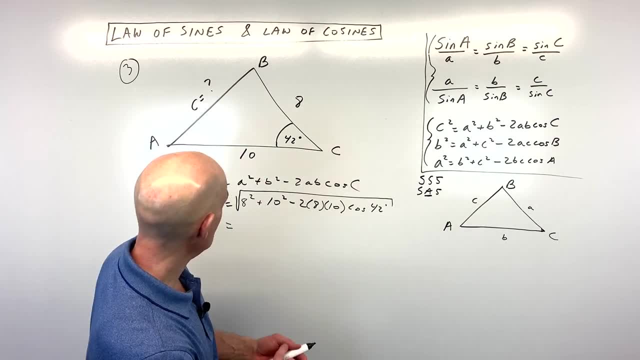 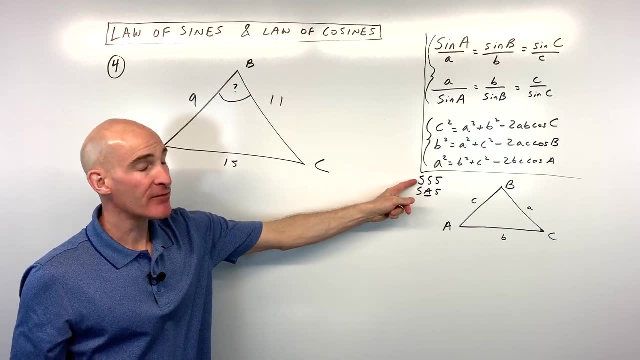 Again, make sure your calculator is in degrees, So that comes out to about 6.7, and you've got that missing side. Okay, example number four: This is the case where you have three sides- side, side, side- and you wanna solve for a missing angle. 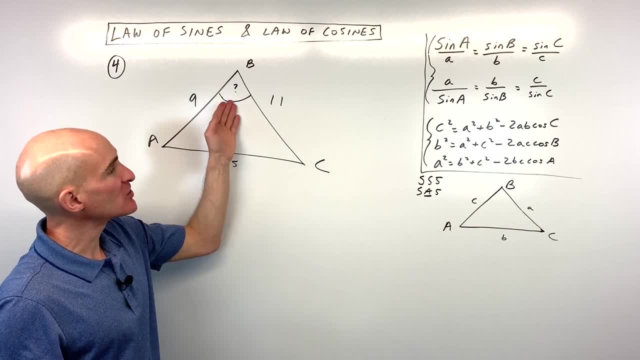 In this case, we're trying to solve for angle b. So what we're gonna do, since we're trying to solve for angle b, let's use this middle equation, where we have side b but not angle b, and let's write that out. 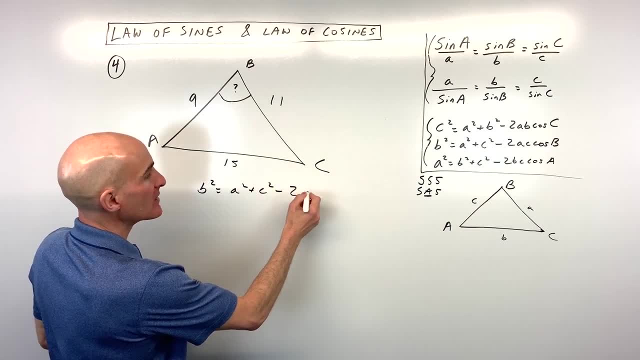 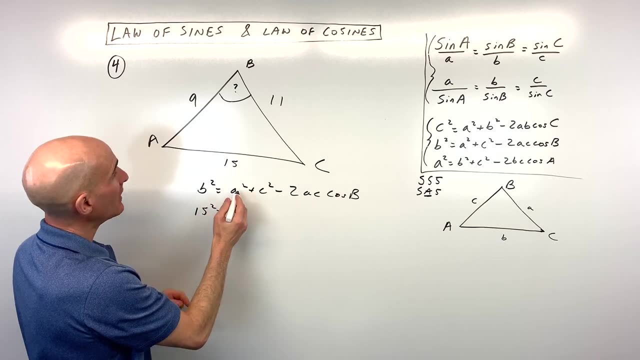 So we've got b squared equals a squared, plus c squared minus two. ac cosine angle b. Okay, b is the side across from angle b, That's 15 squared. a is the one across from angle a, That's 11 squared. 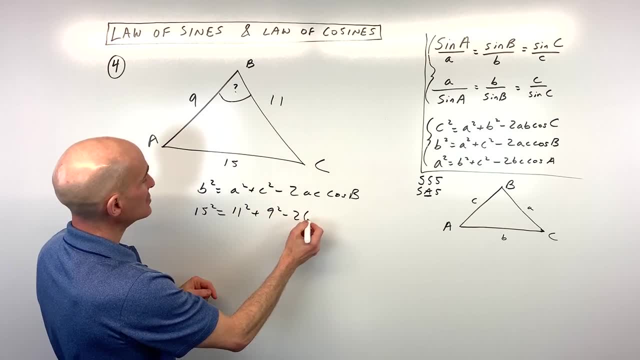 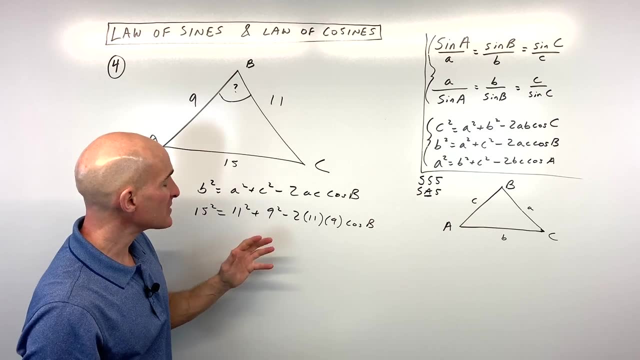 c is the one across from angle c. That's nine squared minus two times 11 times nine times the cosine of angle b. Now, sometimes students make a little bit of arithmetic errors when they're trying to solve for angle b here. So let me see if I can explain this. 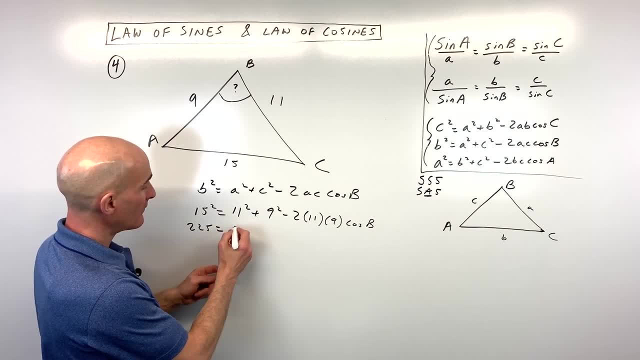 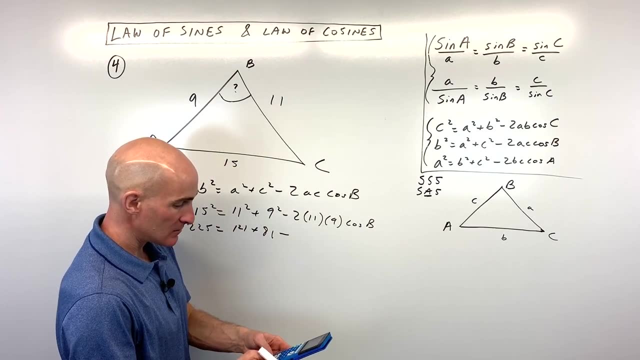 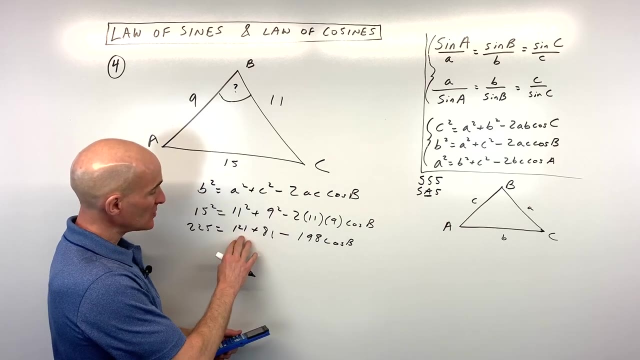 Let's go ahead and simplify a little bit here. We've got 225.. We have 121 plus 81 minus. let's see two times 11 times nine, which is 198 cosine angle b. Now what students sometimes do, 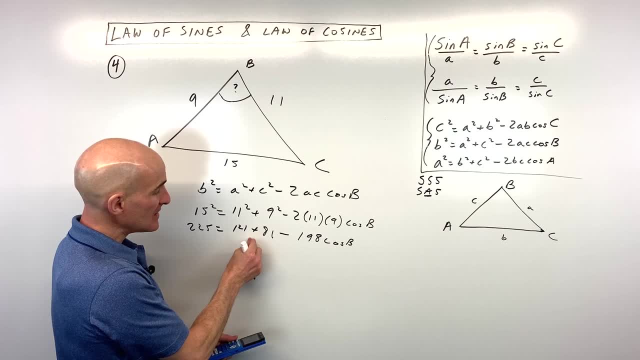 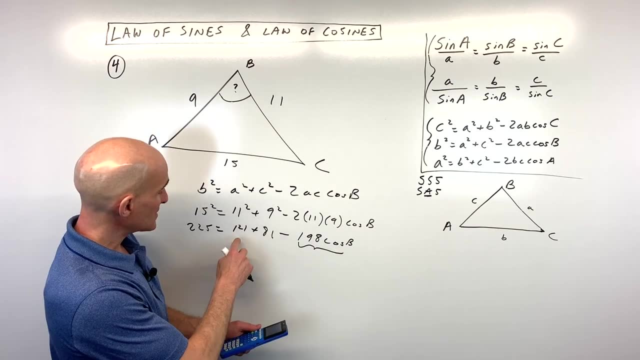 is, they try to combine these numbers here. You can combine these, but you really can't combine with this, because this 198 is multiplied by cosine of e. This is like all one group. So what we're going to do instead is we're going to subtract the 121. 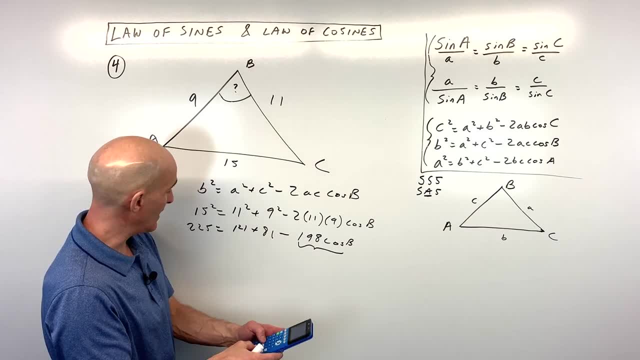 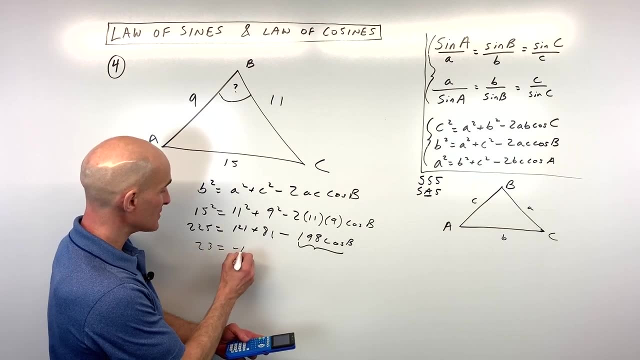 and we're going to subtract the 81. We're going to get them to this left side of the equation, So let's do that now. So 225 minus 121 minus 81. So now we're at: 23 equals negative 198. 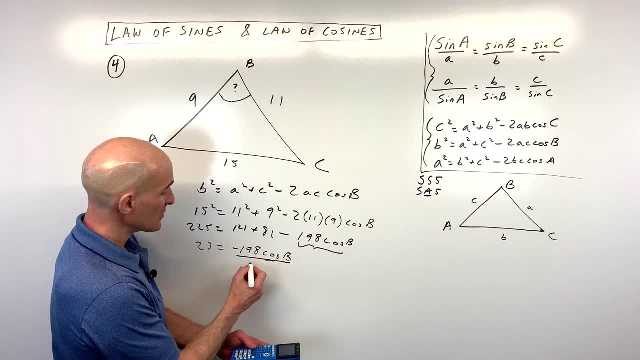 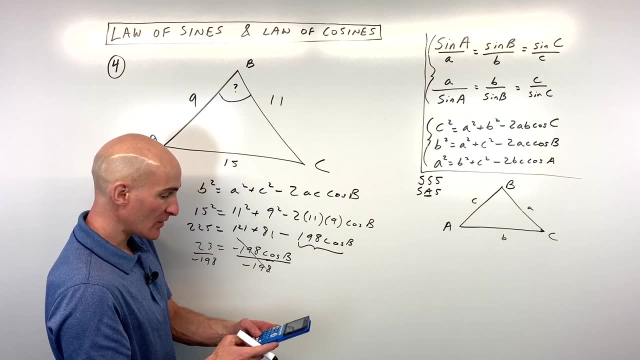 times the cosine of angle b. We want to get cosine b by itself, so let's go ahead and divide by negative 198 to both sides And let's see what that comes out to. Okay, so we're looking at about negative .116,. 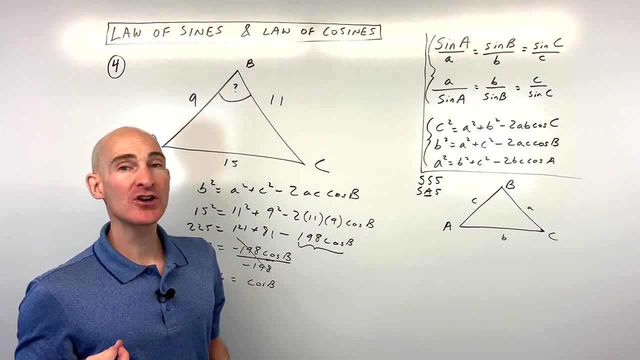 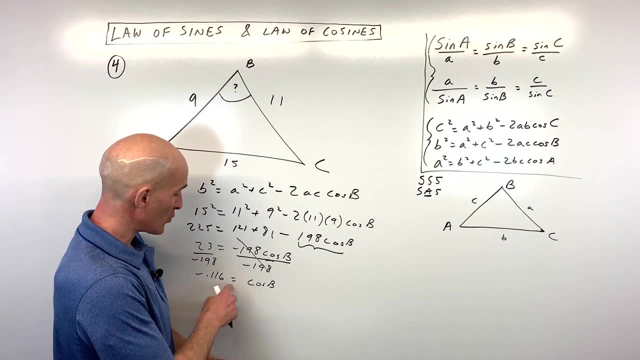 equals cosine of angle b. Now remember, whenever you're solving for the missing angle, that's when you want to do the inverse sine or inverse cosine, inverse tangent, like that. So to solve for angle b, we're going to take the cosine inverse of negative .116.. 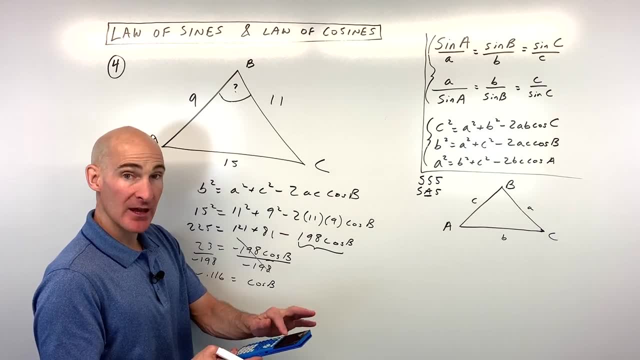 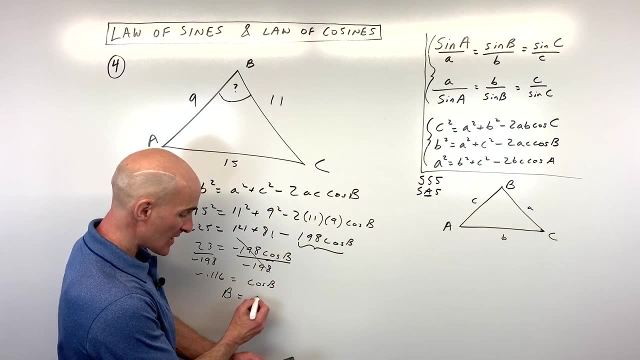 So let's go ahead and do that. And what I tend to do is I tend to, on my calculator, use the previous answer key, so I take that long decimal so I get a little bit more accurate answer. So it looks like angle b. here is approximately 96.7 degrees.